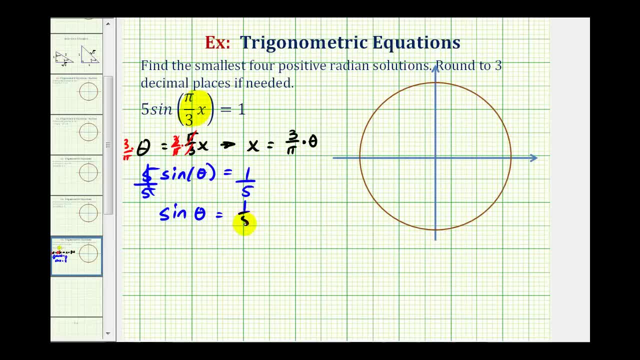 So we have: sine theta equals one fifth. We should recognize that having a sine function value of one fifth is not a value that we'll find on the unit circle or using reference triangles, So we'll have to use the calculator to help us solve this equation. 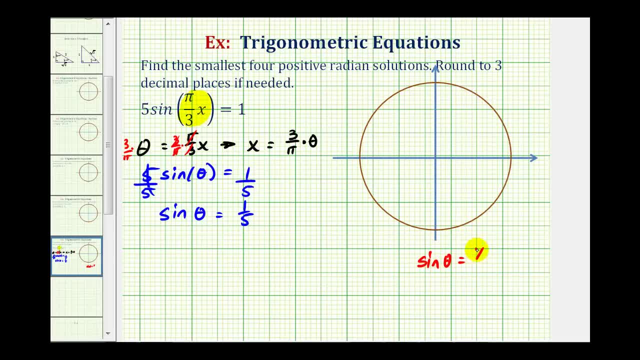 But also, since sine theta equals y divided by r and the sine function value is positive, we should recognize that y has to be positive and therefore our solutions must be in the first or second quadrants where y is positive and therefore the sine function value would be positive. 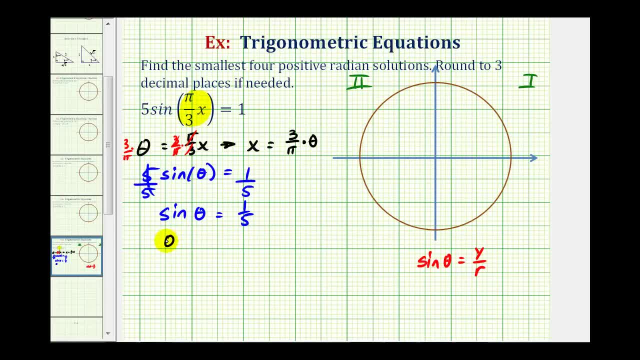 Next, since sine theta equals one fifth, that means theta would be equal to arc sine or inverse sine of one fifth. So now we'll go to the calculator to help us find our first solution. It's important to make sure that we are in radian mode. 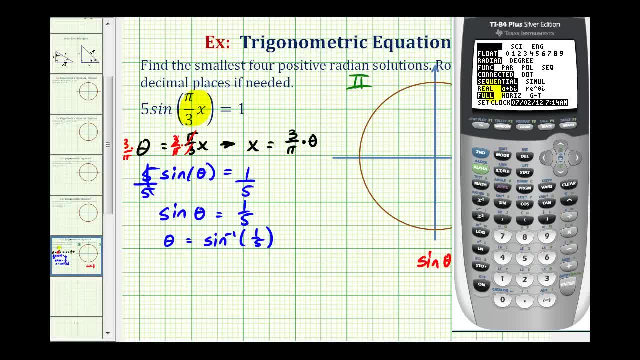 So I'll press the mode key. Notice how we are in radian mode. So we'll go back to the home screen, Press second sine one fifth- close parenthesis enter Because we're asked to round x to three decimal places. and this is actually theta. 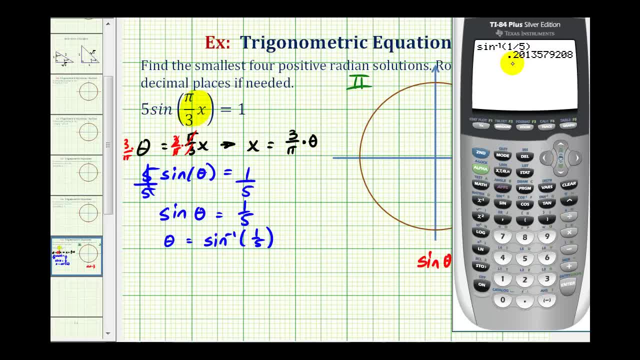 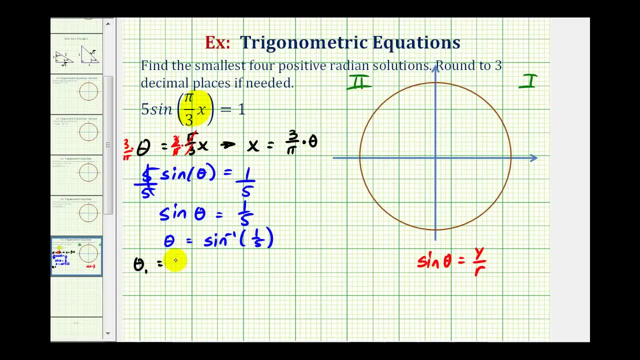 We're going to round theta to four decimal places to hopefully to avoid any rounding errors when finding x. So we'll have: theta equals zero point two, zero one four. So we'll call this theta sub one. Now let's go ahead and sketch this angle. 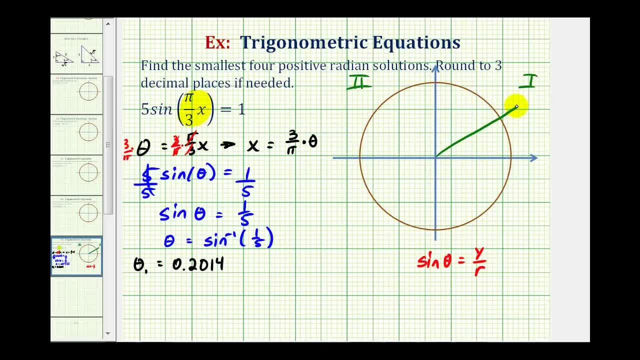 in the first quadrant. Let's say this is the terminal side and this is the angle: zero point two, zero one, four radians. Well, because sine is also positive in the second quadrant, if we sketch a reference angle of zero point two, zero one four in the second quadrant, 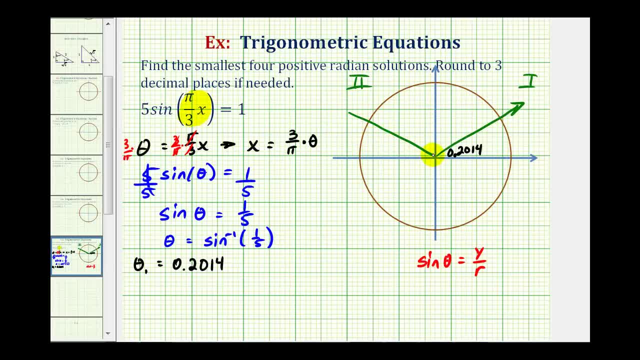 we can also determine a second solution. So again, if this reference angle is zero point two, zero one four, this angle that terminates in the second quadrant would also have the same sine function value. So this first angle was determined on the calculator, and then to determine this angle, 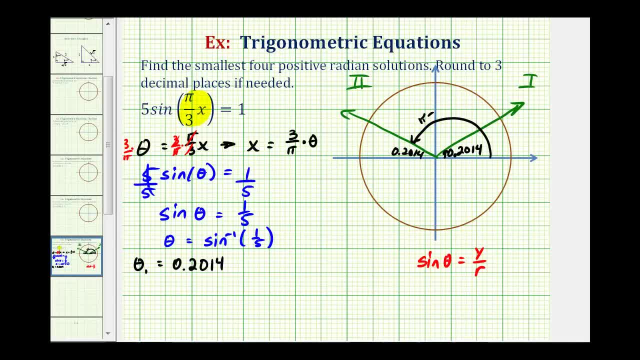 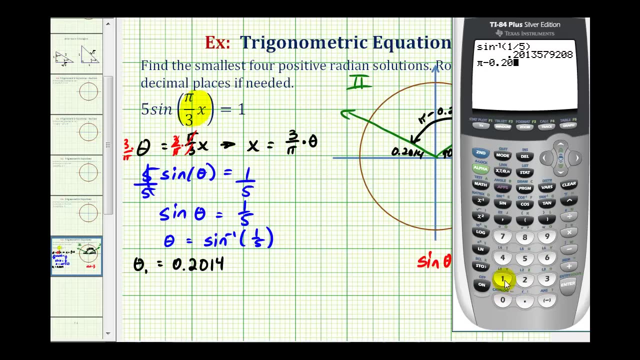 we would take pi radians or half a rotation and subtract the reference angle to determine this angle in the second quadrant. So let's go ahead and do that. We would have pi radians minus zero point two, zero one four. So we'll call this theta sub two. 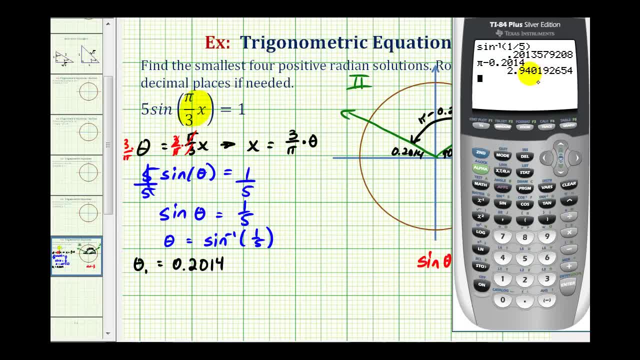 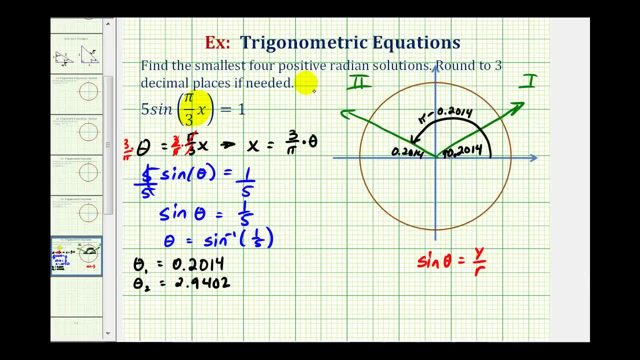 It'll be approximately two point nine, four zero two, Because we're looking for the four smallest positive radian solutions. we need to find two more solutions here, Which means the next two solutions would be coterminal with these two angles. So for theta sub three, 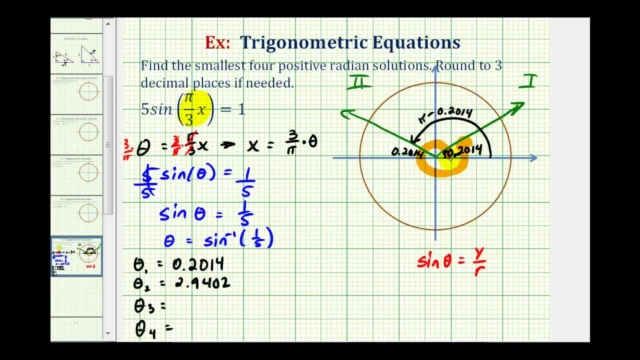 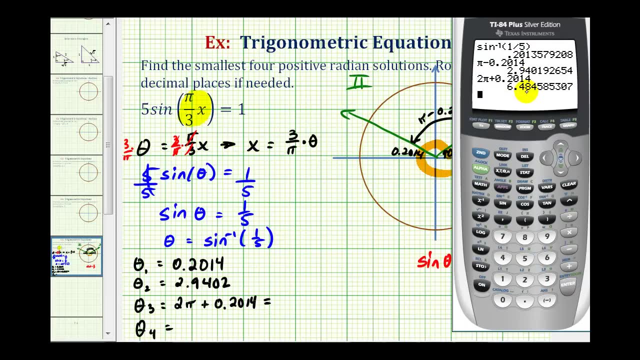 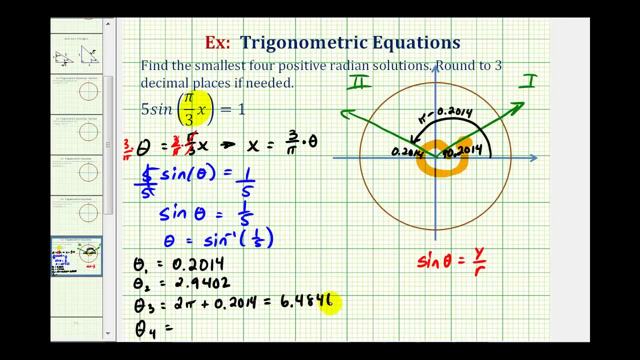 we would have two pi plus zero point two, zero, one, four, Which will be approximately six point four, eight four six, And then theta sub four would be coterminal with this angle here. So we would have two pi plus two point nine, four, zero, two radians. 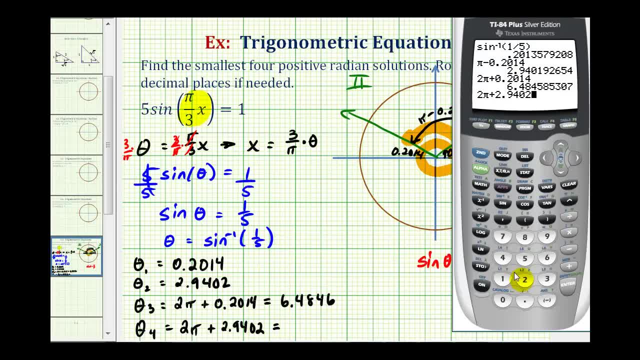 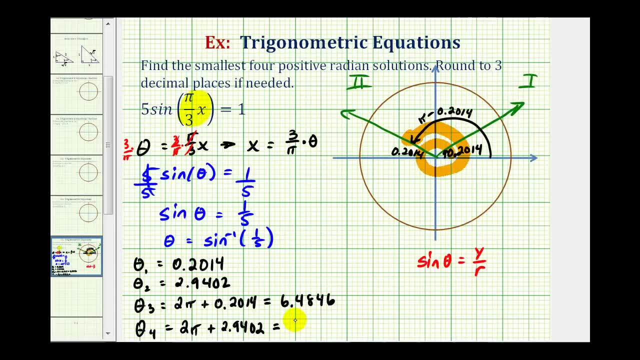 Which is approximately nine point two, two, three, four. But we're not done now. Remember our goal is to solve for x, not theta, Where x is equal to three divided by pi times theta. So we'll have to take these values here and then multiply by pi over three. 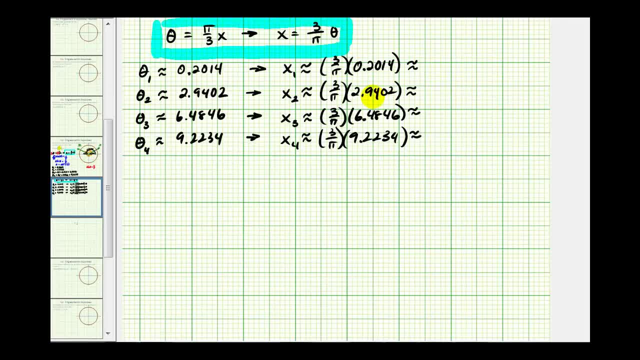 And we'll do that on the next slide. So our initial substitution was: theta equals pi divided by three times x. If we solve this equation for x, we have x equals three divided by pi times theta. So these are the values that we found for theta, So multiply. 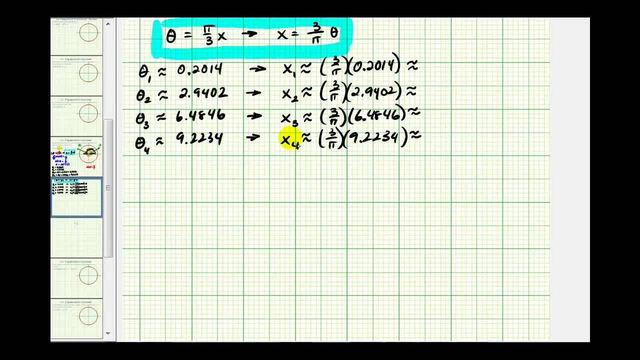 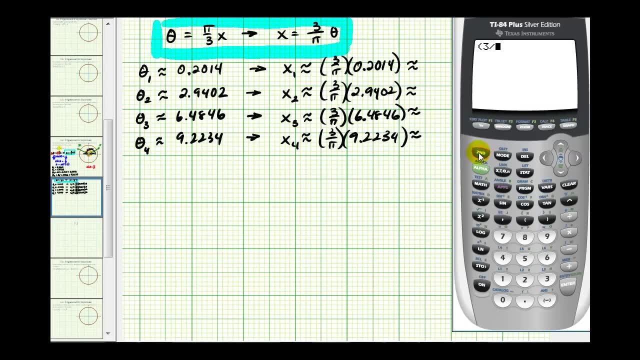 each of these by pi divided by three, to find the approximate values of x for the original trig equation. So let's go ahead and do that. And the directions do say around to three decimal places. So x sub one is approximately zero point one nine two radians.